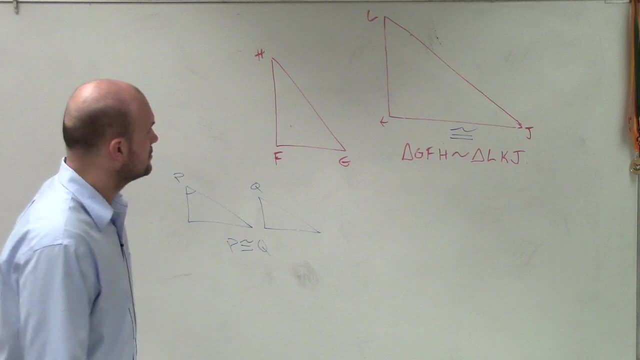 what are the things that go with it? OK, G, J, GFH, GFH, OKJ, OKJ, OKJ. That's what it's going to be. What's that on the corner? That's a K. 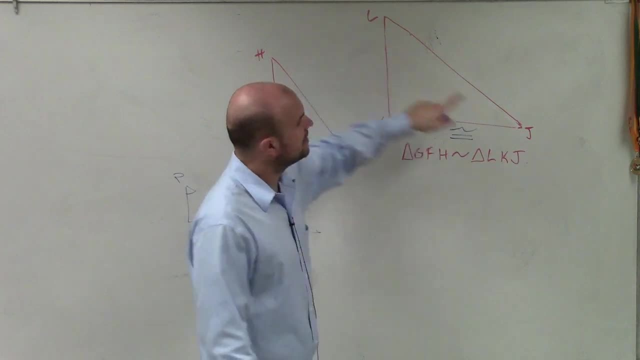 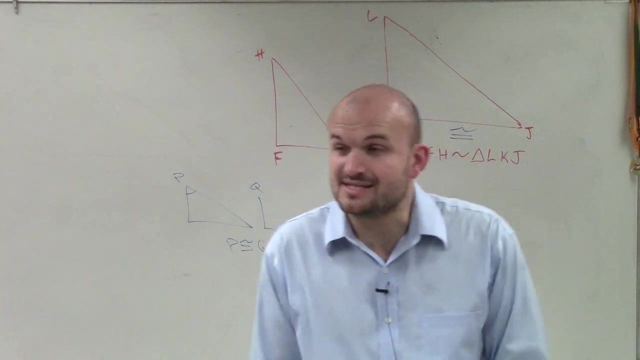 That's a K, That's another K. Shut up K, L, J. All right Now in this case. so we have this P and a G. We can say that those are corresponding to each other. They're congruent, but they're the exact same. 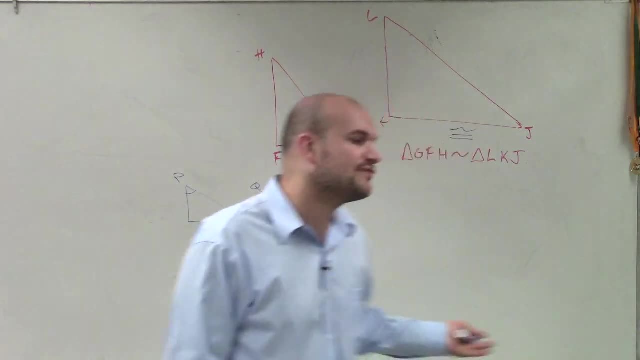 The reason why? because they're in the exact same shape and position for both triangles. Well, what I want you guys to understand in this case, when we're dealing with similarity, we're going to have corresponding parts as well. So the corresponding parts in this triangle. 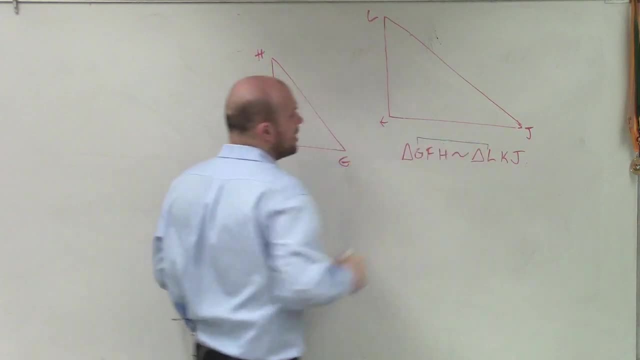 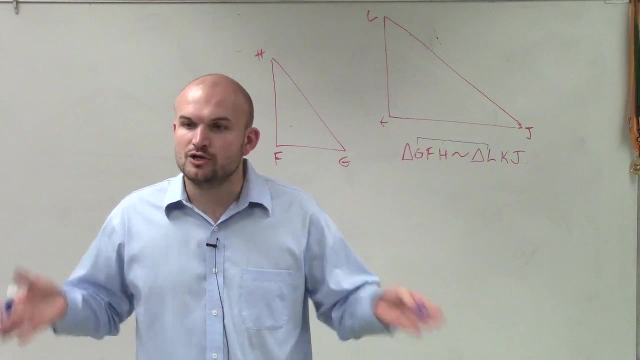 we can do the same thing by going back to our similarity statement. all right, Because, remember, when you do a similarity statement, just like when you did a congruency statement, you have to label them in the same order, all right. 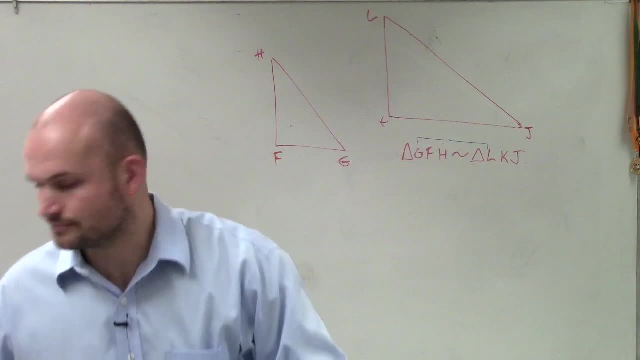 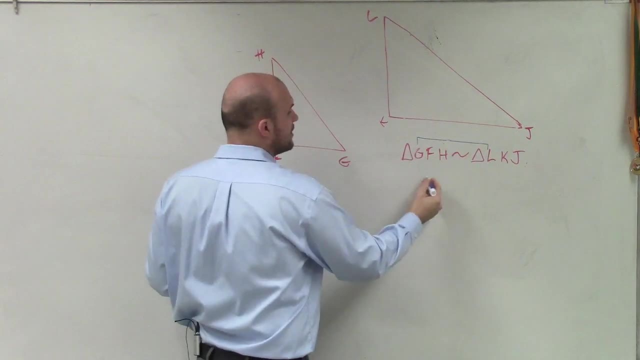 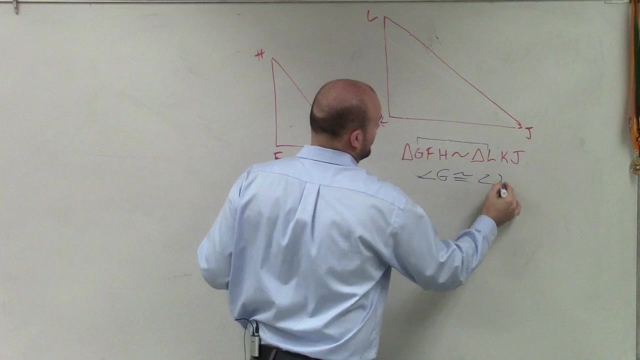 You have to label them in the same order So I can say that angle G is congruent. It's congruent to angle L. So what I'll write is the measure. I'm going to say: angle G is congruent to angle L Because remember, 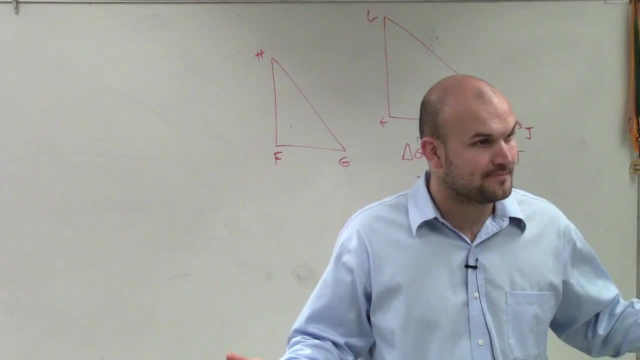 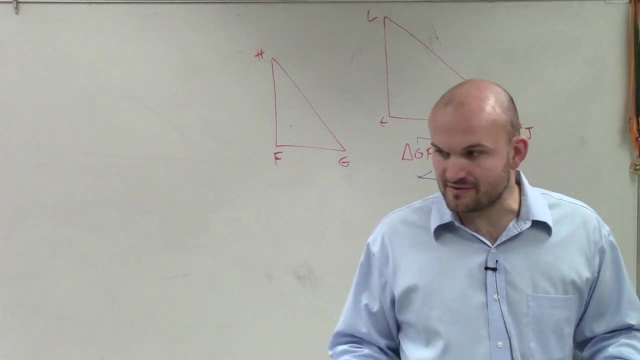 when we talked about similarity, angles can be exactly the same, right, They can have the same size or, I'm sorry, the same shape, just not all the same size for all their lengths and everything But the angles. remember we talked? 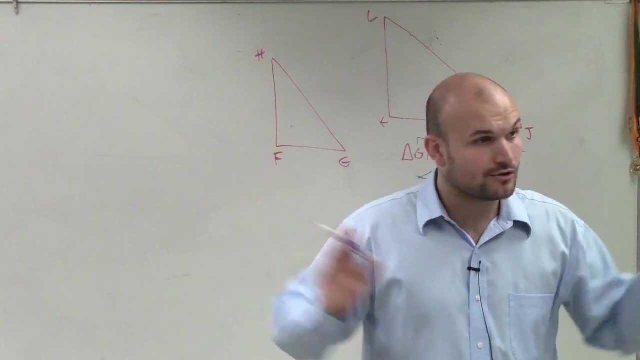 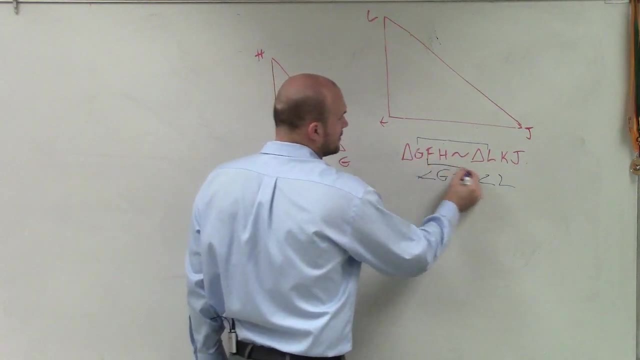 about equilateral triangles, the 60-60-60?. That could be a big triangle or it could be a small triangle, But the angles are still going to be congruent to each other. So I can say angle G is congruent to angle L. 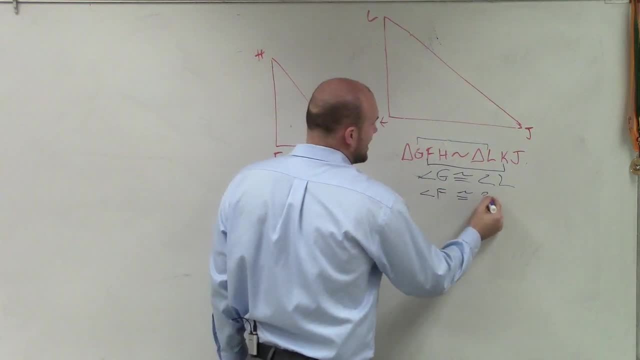 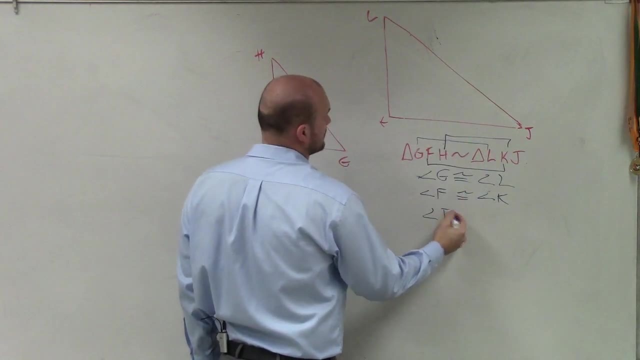 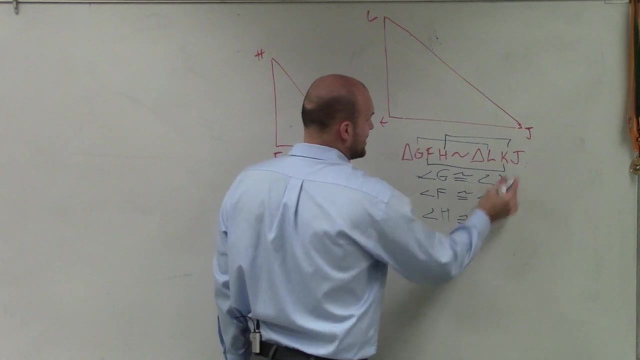 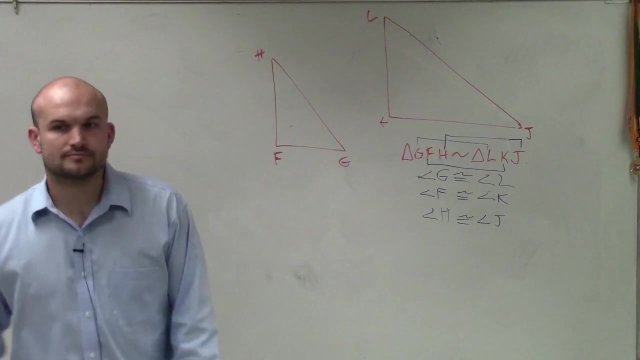 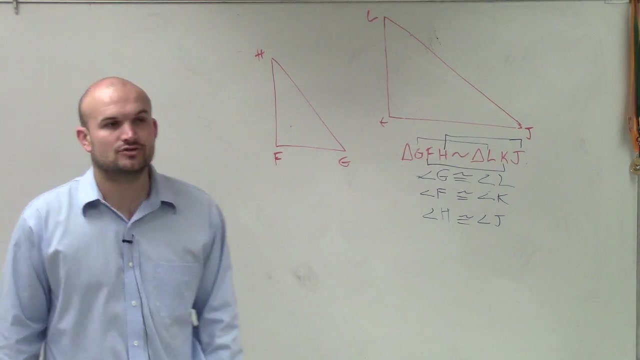 Angle F is congruent to angle K And angle J is congruent, or angle H is congruent to angle J. Angle A- G is congruent to angle L, Angle F is congruent to angle K And angle H is congruent to angle J. 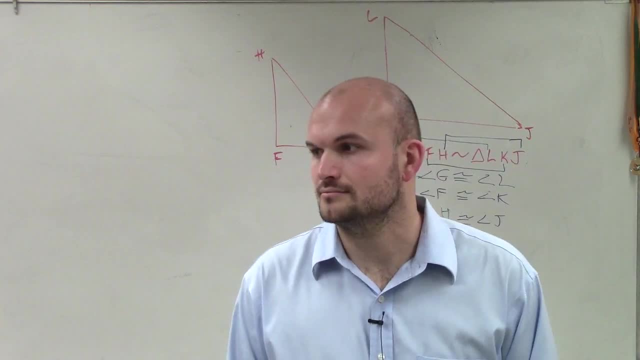 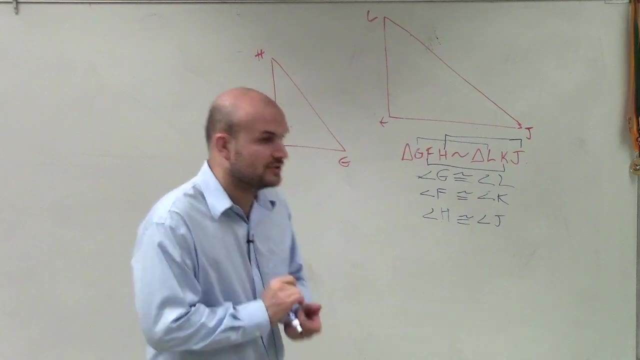 OK, Well, that's what we're going to be doing in just a second. Did we already know that? Yeah, we did. You should already know that, So there should be a review. So now what we're going to be talking about. 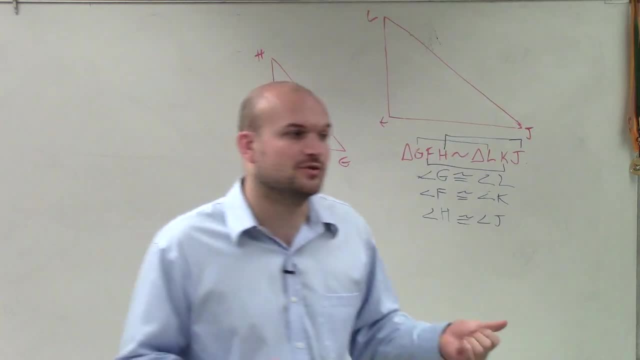 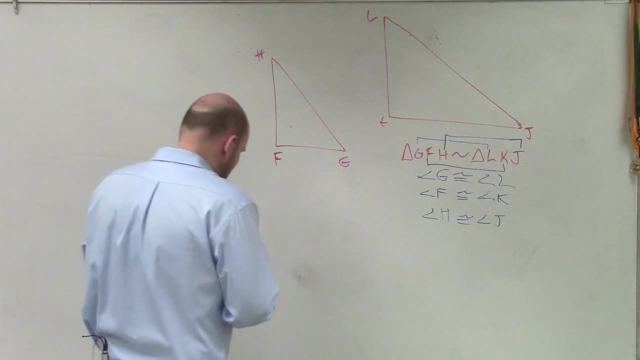 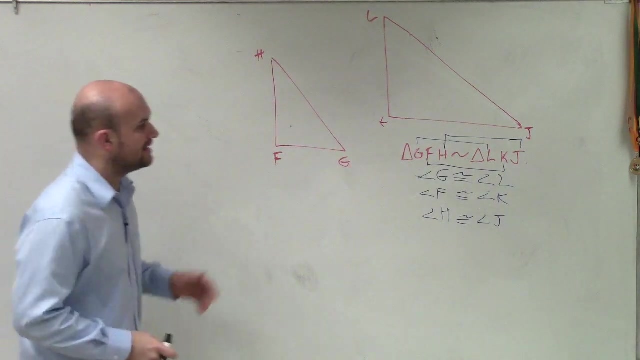 is now setting up a proportion, Because what actually the question asks you, what we want to be able to do, is not only set up corresponding sides or angles, But also set up proportions. So what I want you guys to understand or recognize with this problem is if G is corresponding to L. 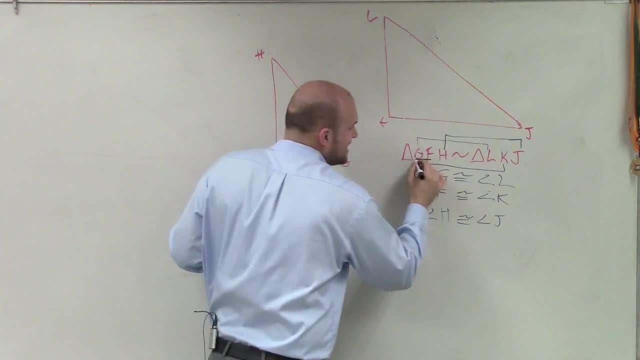 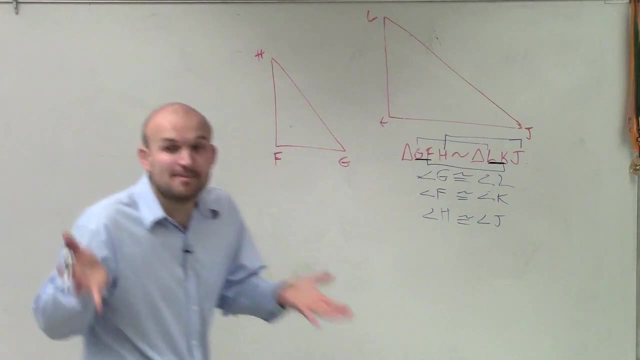 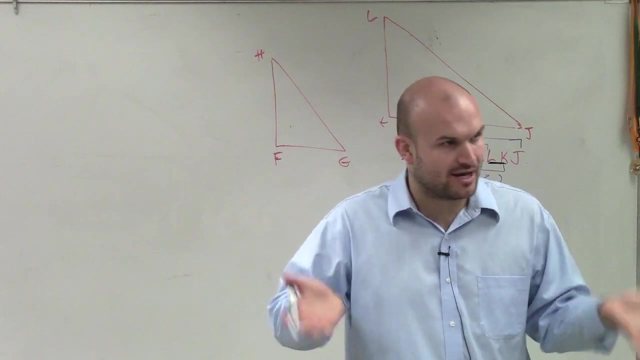 and F is corresponding to K. does it make sense then for me to say: GF is similar to LK? Does that make sense? But it's similar, It's not congruent. right Before, In congruency, we'd say: this is equal to that right. 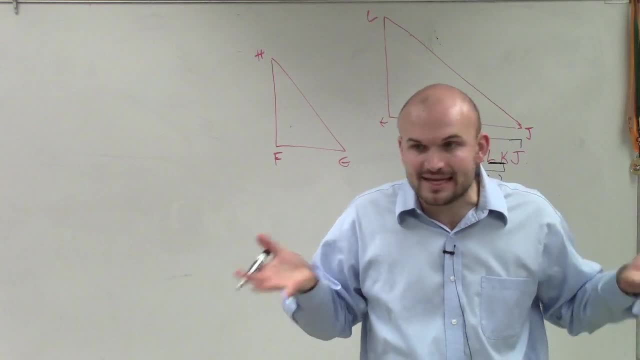 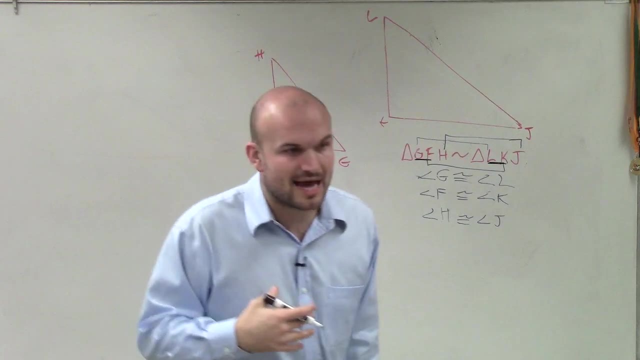 And we'd say they are congruent. But now we're talking about similarity. They're not equal to each other anymore, Or they don't have to be equal to each other, So now they're similar. So what we want to do in this class? 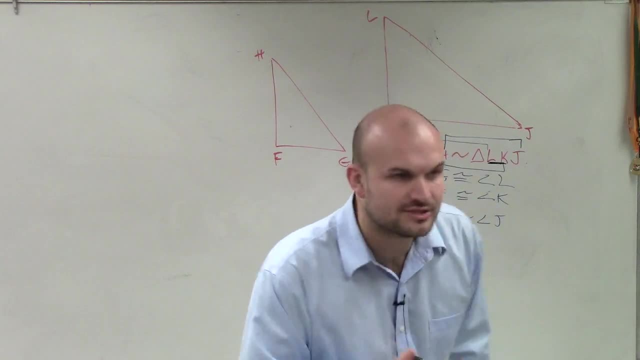 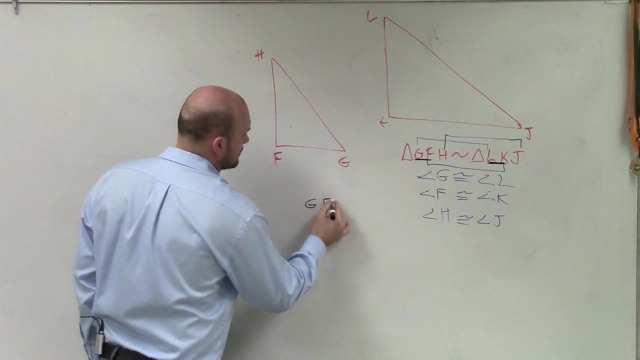 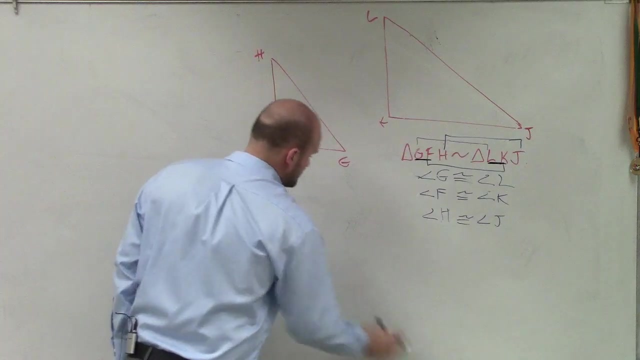 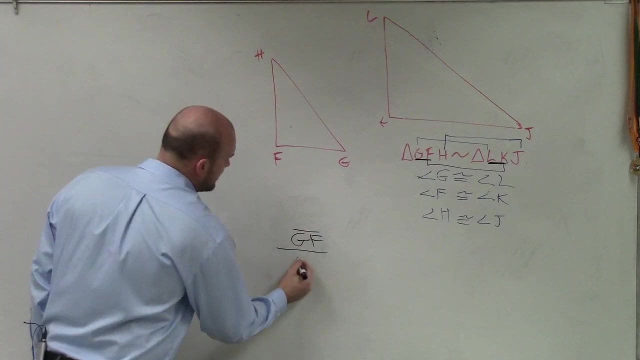 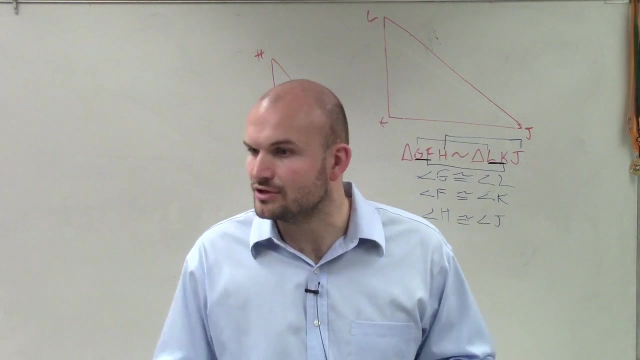 is compare them using a ratio. So what I can say is G8 or GF. Let me write it over here So I could say line GF divided by LK, That is one ratio of the two sides. right, Because those are similar sides, correct? 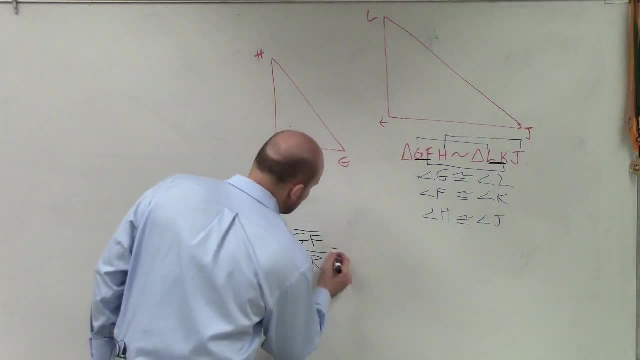 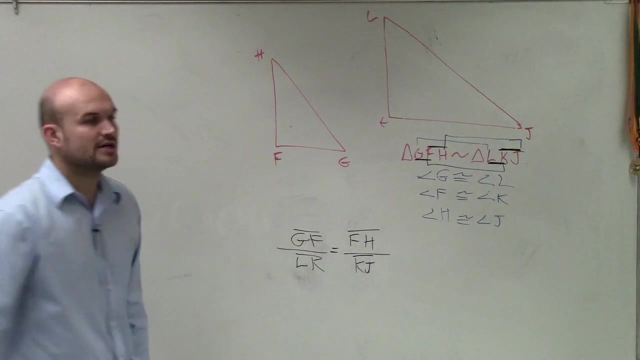 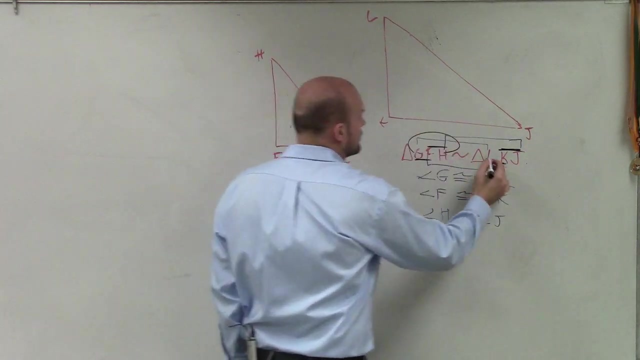 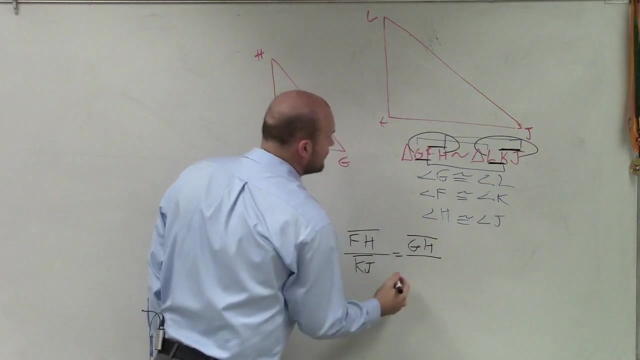 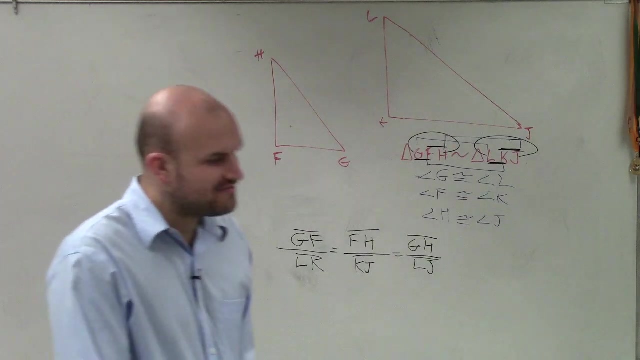 Would everybody agree they're similar sides. Well, that ratio is equivalent to this ratio: FH over KJ- Did you guys agree with that? And that ratio is equivalent to this ratio to GH over LJ. So what you guys want to make sure you have for this.